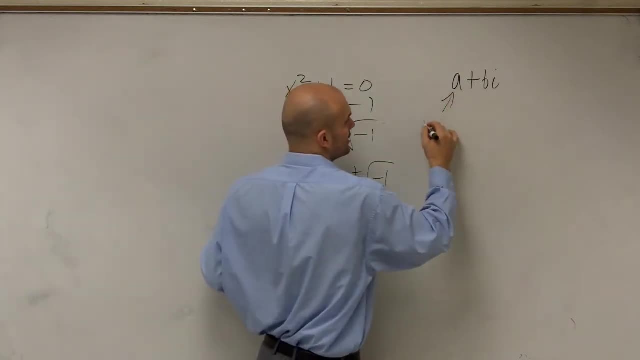 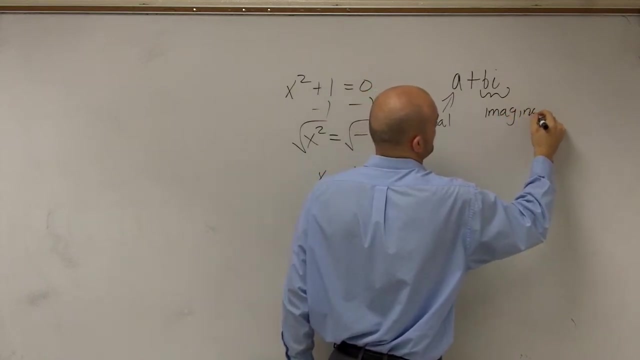 We had to write them in that form where a is your real part and then bi is your real part, And then we had to write them in that form where a is your imaginary part. all right, So complex numbers when we were adding, subtracting, multiplying. complex numbers. 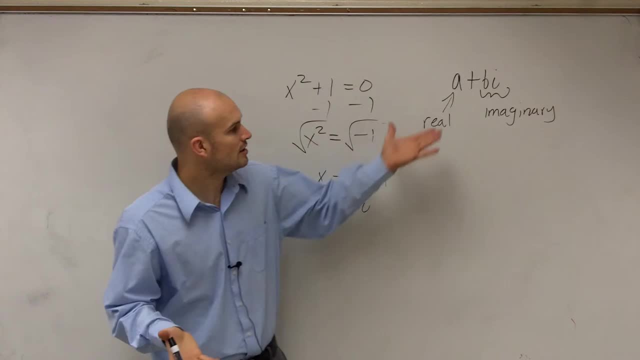 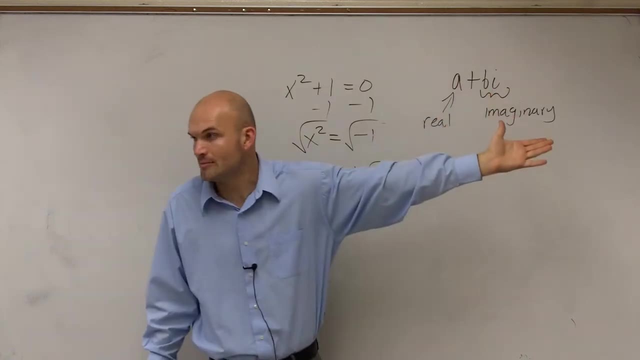 and all that kind of stuff. what we found out is, when we write a complex number, we always have a real part and then we have an imaginary part. all right, And dealing with your- i is obviously dealing with your imaginary part of that. 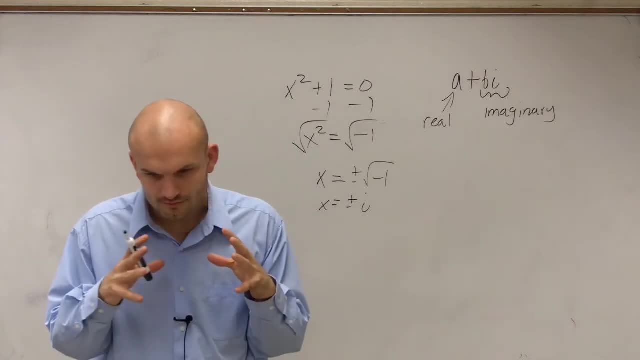 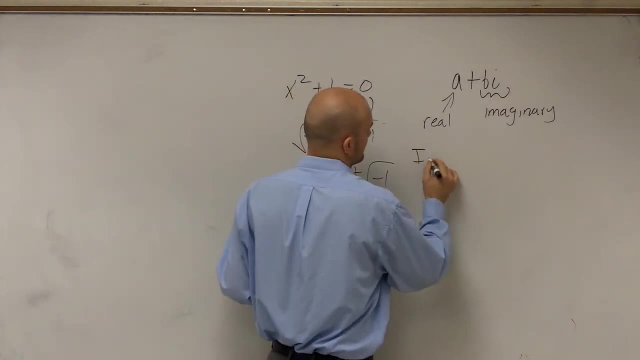 So what I want to go through with you is what we call the complex conjugate theorem. all right, And what that's going to state is, first of all, if a plus bi is a factor, all right. If a plus bi is a factor of your polynomial. 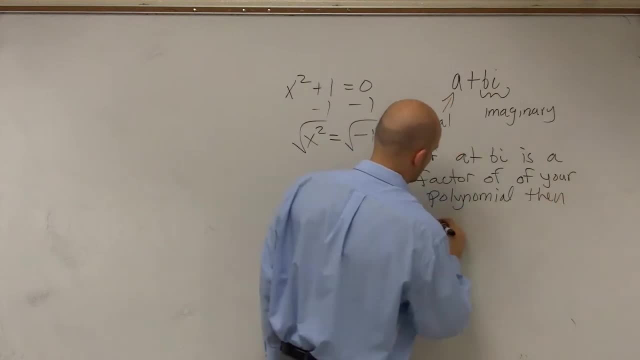 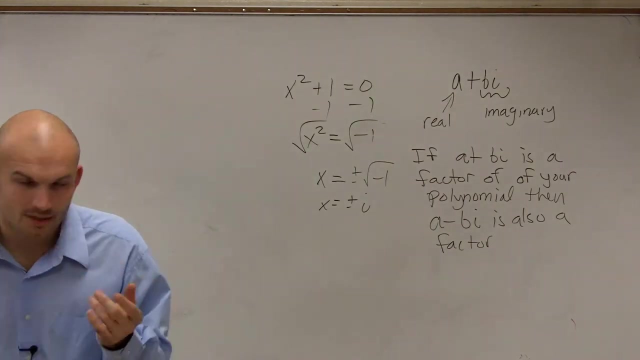 then a minus bi is also a factor, all right. So you guys are going to want to make sure you guys have have that written down, all right, And notice that there, that where that's when a can be any real number. 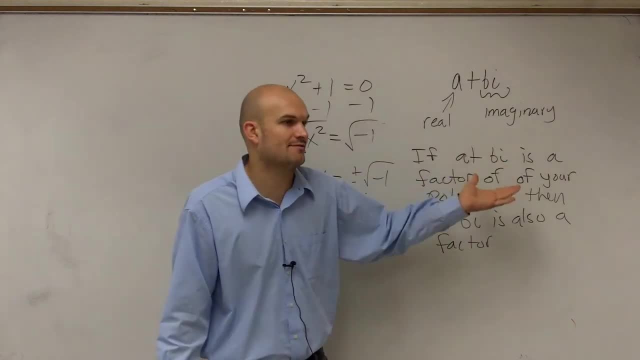 and then b cannot be zero, because obviously if b was zero, then you wouldn't have an imaginary number, okay? So this is going to be something very, very important for us to understand. So if a plus bi is a factor, so if I say a plus bi is a factor, 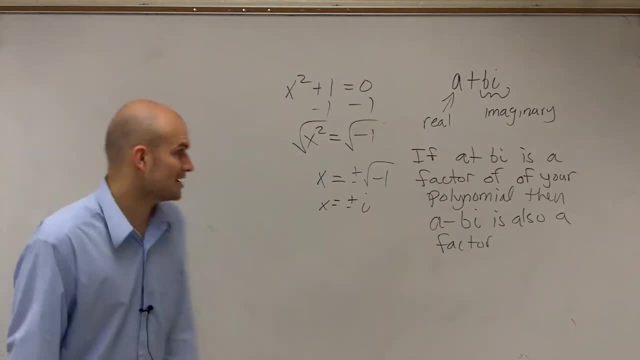 then that means a minus bi is a factor. So let's just kind of go through this real simply then. So if I say one minus i is a factor, then what's my other factor? Okay, all right. What about if I say negative 2i is a factor? 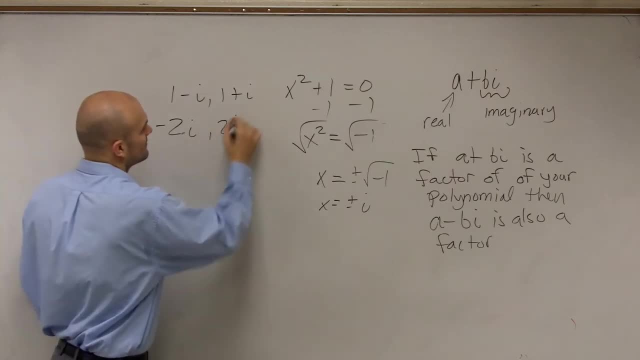 Positive 2i. You guys are too smart. Okay, very good. So that's all we're going to really need to know about the conjugate complex conjugate theorem. But that's good, Good job. So why would I tell you something like that?